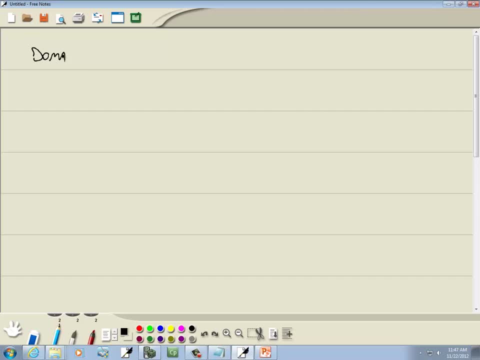 Domain of a function. By default, it's all real numbers except ones that cause a zero in a denominator. Let's take a look at how to find it graphically. By default, it's all real numbers except ones that cause a zero in a denominator. 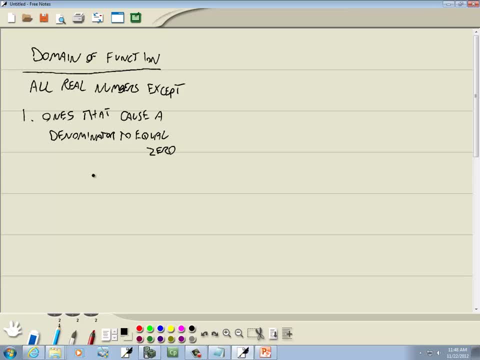 Now we'll add on to this. At the end of this course we'll add a second one. on here In college algebra you add a third one. The second one deals with radicals, with even indexes, And the third one- Actually there's. 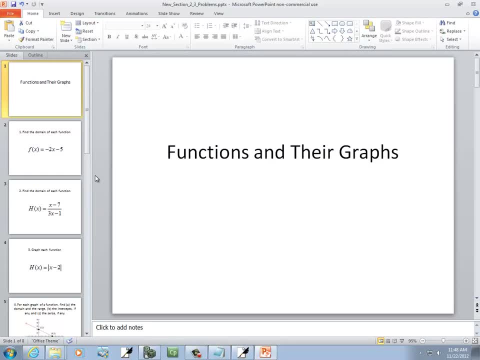 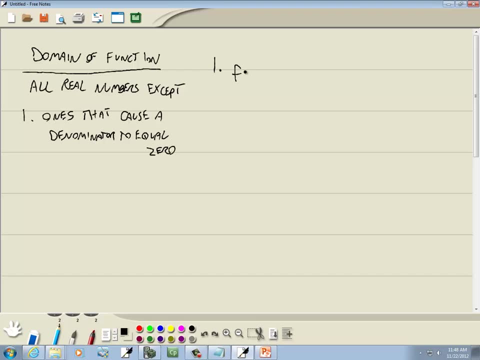 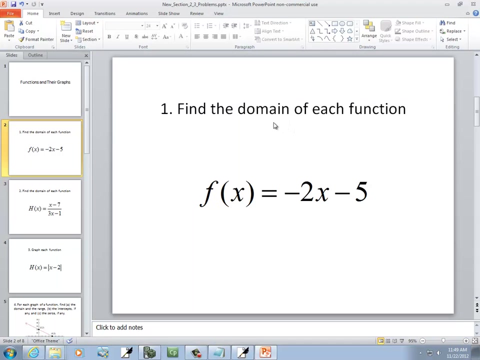 Yeah, the third one's law. so it's just like: why did you number those number one if there's only one? so our first one here we've got: f of X is equal to negative 2x minus 5, and the instructions say: find the domain of each function. well, by default it's all world. 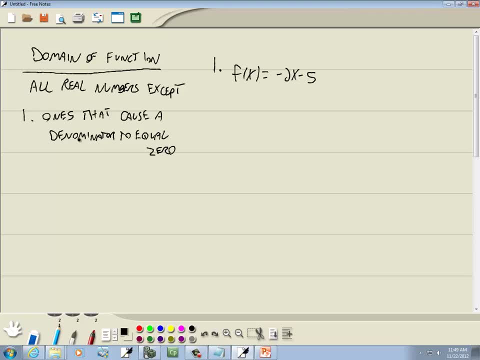 numbers, except for ones that cause the denominator equals zero. now, to have a denominator means you have to have a fraction. well, if we don't have a fraction, then by default our domain is all world numbers and we'll write it as negative infinity, positive infinity. parentheses run like that. that's interval. 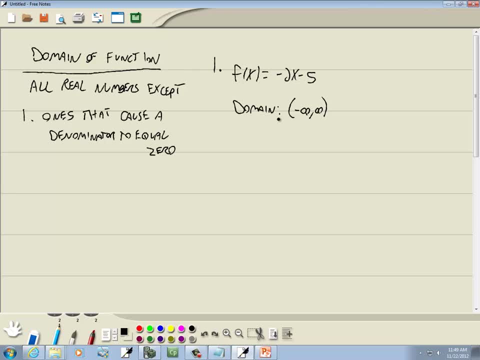 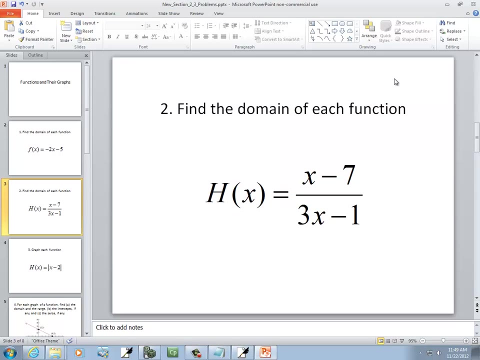 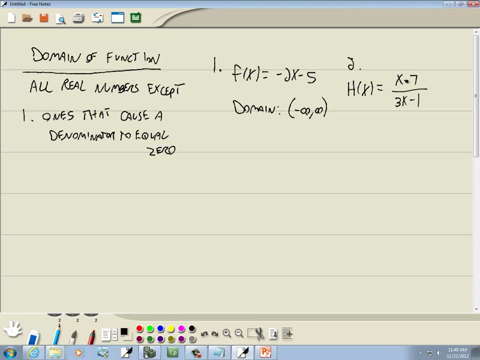 notation- very short way to write all world numbers. let's take a look at one that has a fraction. if it doesn't have a fraction, it's very easy: H of X is equal to X minus 7 over 3x minus 1. if you have a fraction and you find the domain, what? 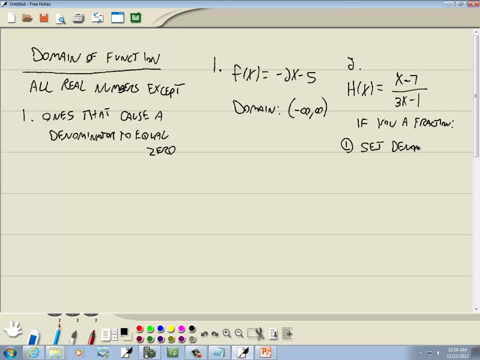 we're going to do is we're going to set the denominator equal to zero and solve. so set denominator equal to 0 and solve. so we'll take the 3x minus 1, set it equal to 0, this is a linear equation, so I take negative 1 over, becomes a. 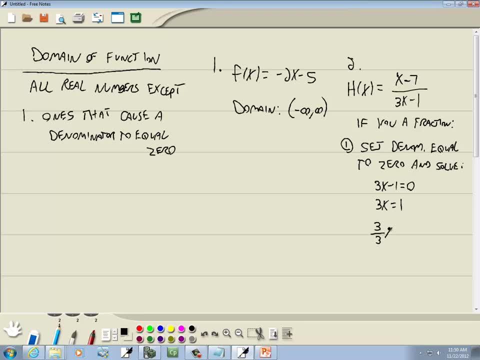 positive 1, divide both sides by 3. arees would cancel and we got. X is equal to 1. 3rd, now, this is a value thatura I'vebeen- Bean addition: triple Зание markЗвызвREEент, bishop of the right hand. الا индемная впередпесケ а數ентилимов. 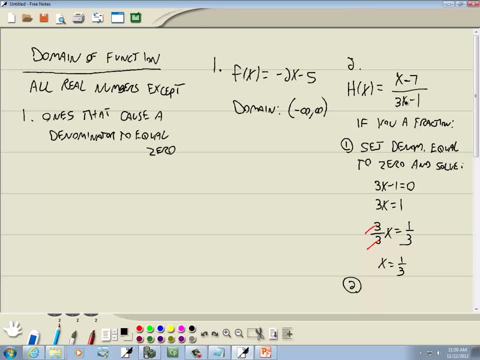 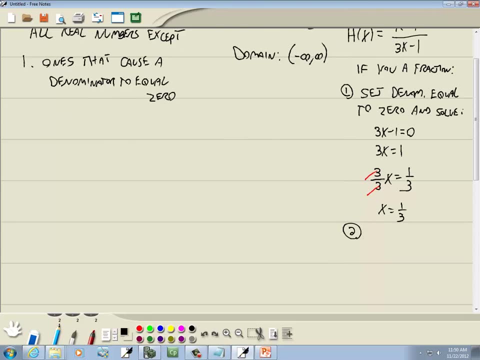 causes problems. If I put one-third in here, we've got three times one-third, which is one. One minus one gives you zero. You can't have a zero in a denominator, So our second step is to put a slash through the equals. 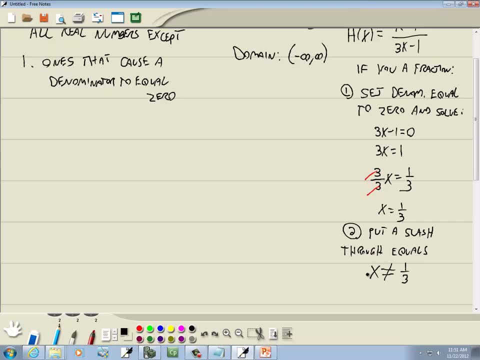 So x cannot equal to one-third. It can be every other number, but it can't be one-third. Now if you prefer to write an interval notation, how you'd write that this is negative infinity to one-third union. that's what that u represents. 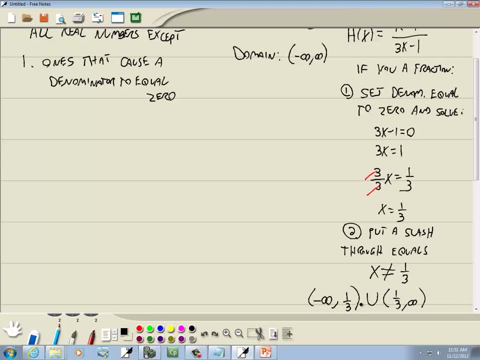 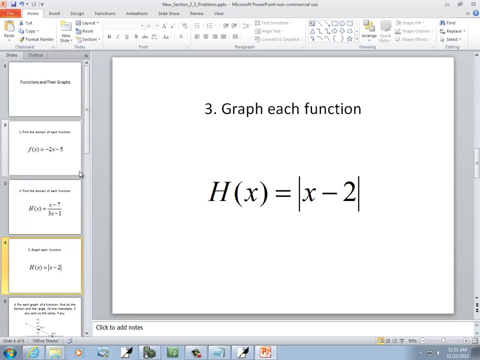 one-third to positive infinity, with parentheses on everything. So that's how you write the same thing in interval notation. Personally, I'm happy with this form, right here. Now next problem: um, what's this? to graph a function? And uh, they're just trying to point out here that it's 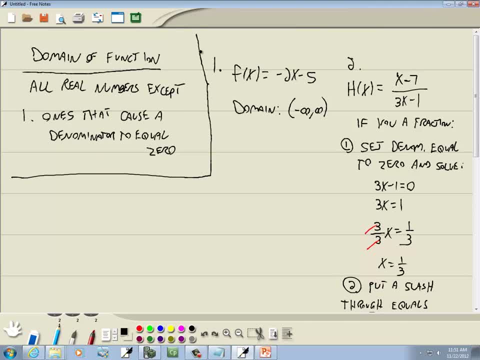 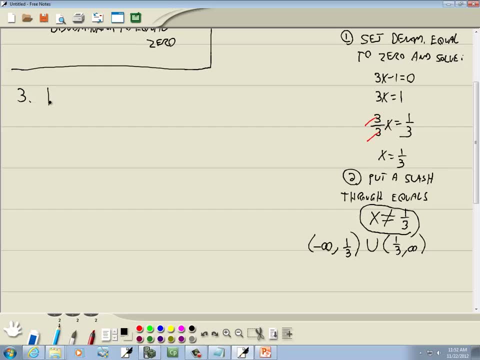 kind of the same as before. So we've got: h is equal to absolute value of x minus two. You'll get used to um function notation being interchangeable with your y. So this is just: y is equal to x minus two. y is equal to absolute value of x minus two. 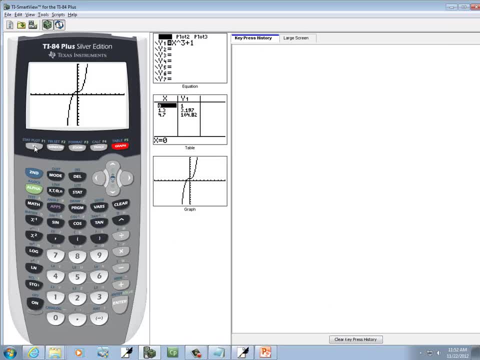 So let's graph this. Press clear there. Or well, press y equals Press clear To get the absolute value. That's under your math button. So press math Right arrow to num. abs is already selected, So I'll press enter on it. 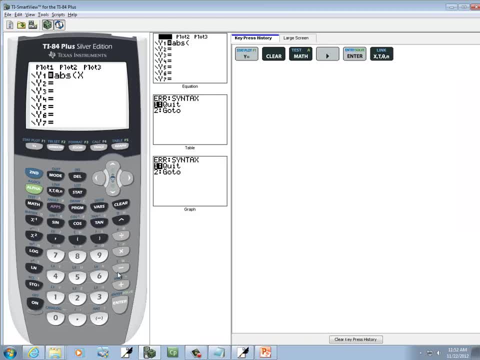 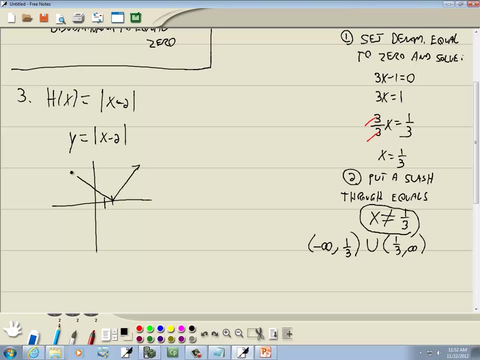 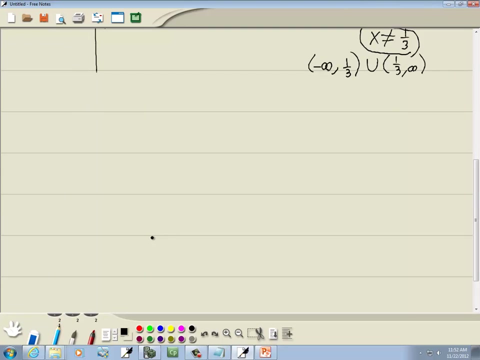 And then we'll put in x minus two. So I'll press my x key minus two And I'll put a closing parentheses And then graph, And that would be our answer. Now, um Domain, Let me uh. 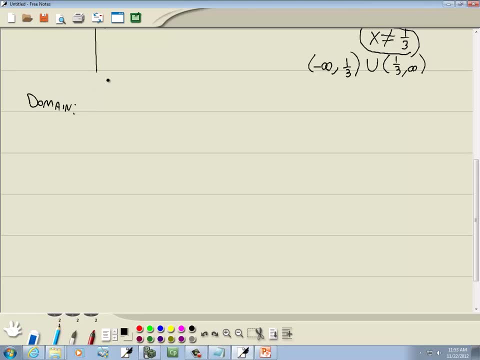 write all these down again. Domain. uh, we saw algebraically, Just uh, for graphically it's the x values. It's the x values Where the graph exists And range is the y values Where the graph exists. 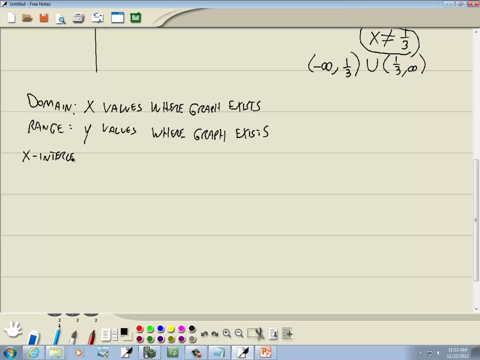 Our x intercept is is where it touches Or crosses the x axis, And our y intercept is is where it the x axis touches or crosses the y-axis. Now there's actually another one. I'll go ahead and write up here. 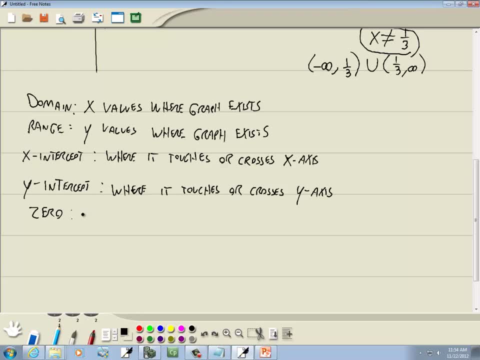 I don't think it's until the next lesson, but it's a zero And this is where it touches or crosses the x-axis. Now, usually this is written in the form of: x is equal to a number. You don't write it in point form like you do the x-intercept. 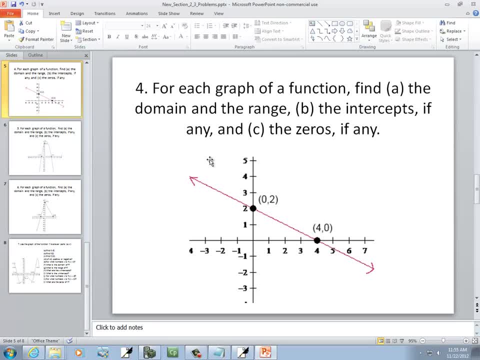 Let me grab a drink here. Oh no, it is a section of zeros. Well, we looked at how to algebraically find a domain, And so now we're given a graph and it's asking us to find the different pieces. 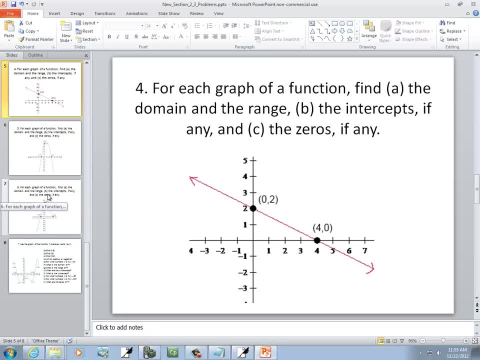 So number four: For each graph of a function, find the domain and the range. Now our domain is the x-values, where the graph exists. Well, if I come up here to the negative two, can I go up or down to find my graph? 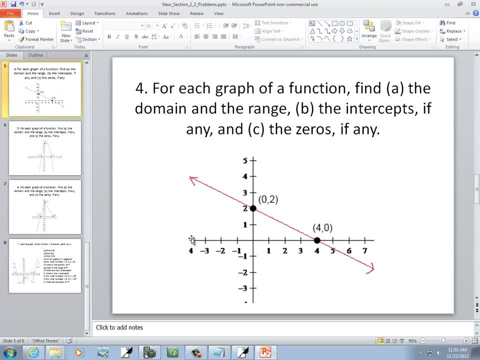 Yeah, I can go up and find it Here. this is negative four, It's cut off. but if I go up to negative four, I can go up and find my graph. Now, this keeps going forever. this graph does. 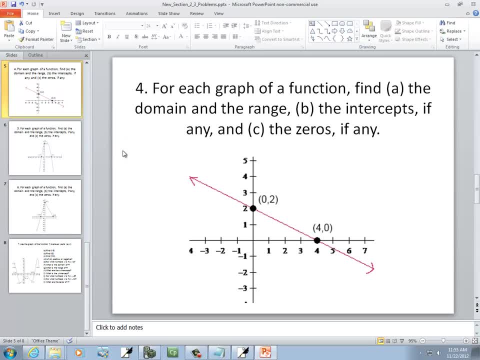 So if I come out here to x equals negative ten, I can go up and find my graph. Train is ear-splitting next. So look, I got it right next door. If I come up here to x equals ten, I can go up and find my graph. 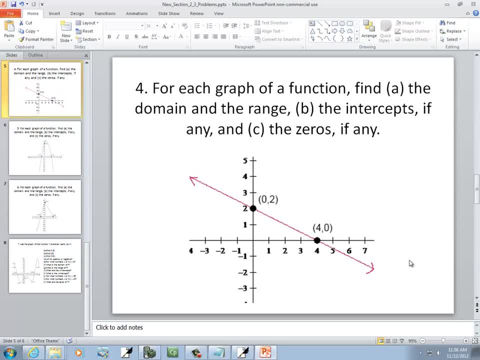 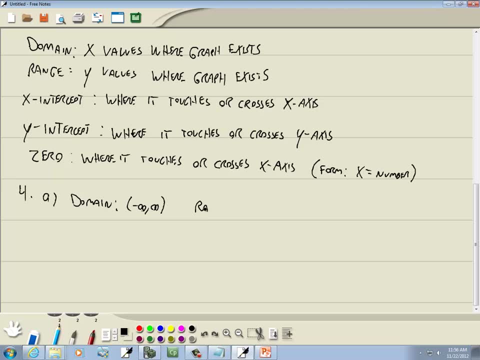 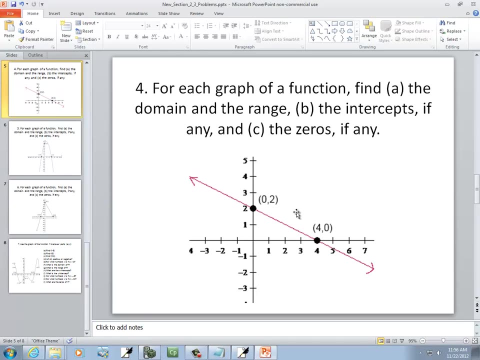 If I come up here to x equals ten, if I go down, I can find my graph. So this actually encompasses all my x-values, which would be negative infinity to positive infinity. Now our ranges are y-values And really the only way you can find range is by looking at the graph. 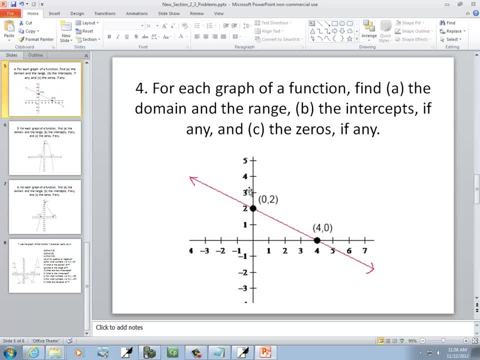 There is no algebraic way like we did with the domain. If I come up to, y is equal to one. the question is: can you go left or right and find your graph? Well, yeah, I can go right and find my graph. 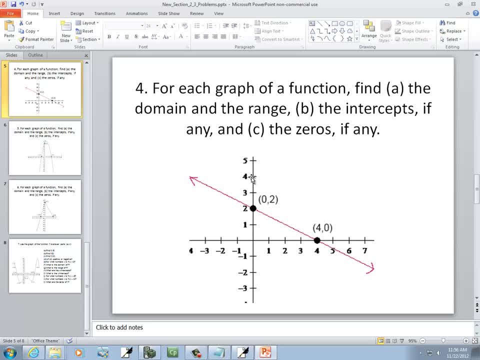 It exists at one. If I come up to y is equal to four, can I go left or right and find my graph? Yeah, I can go left and find my graph If I come up to y is equal to twenty. clear up here. 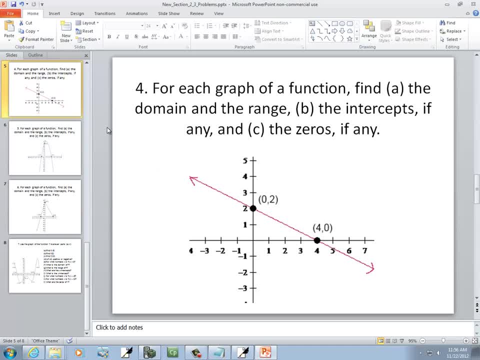 Well, if I go far enough to the left, I will find my graph. because this keeps going like that, So it's slowly going up, so it will eventually encompass all my y-values going up. And this is going down, so it will eventually encompass all my y-values going down. 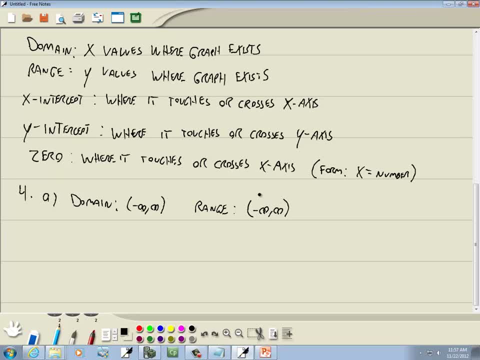 So our range is negative infinity to positive infinity. B, the intercepts. Well, our x-intercept, That's where it touches or crosses the x-axis, which is at four zero. Sometimes people just write four, and I'm happy with that. 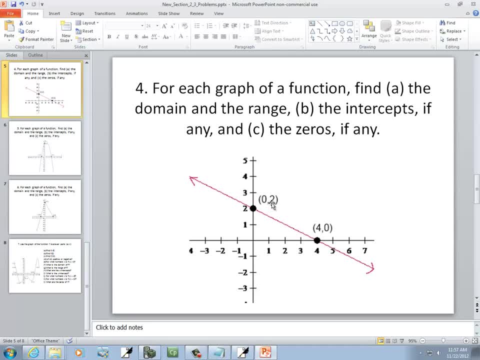 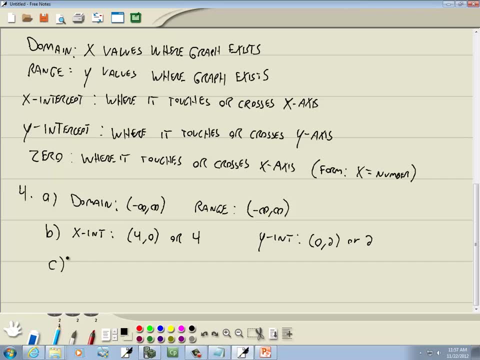 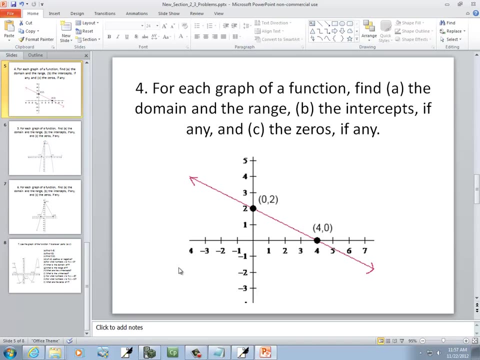 Now our y-intercept is where it touches or crosses the y-axis, which is at zero two. Or, if you want to just write two, I'm fine with that too. Now c is the zeros. Well, zero is just where it crosses or touches the x-axis, which is at four. 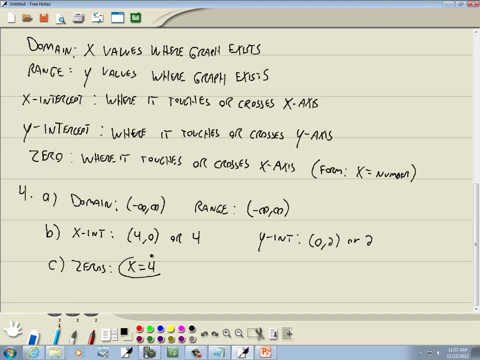 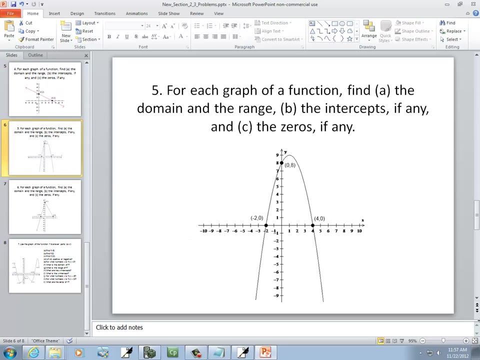 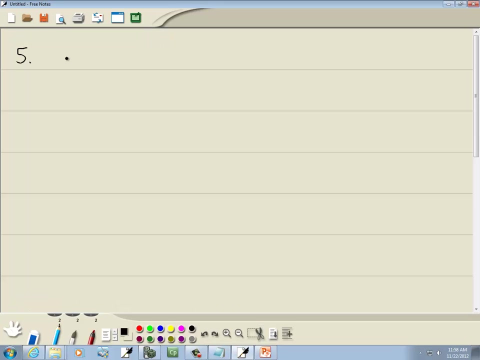 And you write your answer as x equals four. So those would all be our answers for that problem. Let me start a new page here. Same instructions For each graph, find the domain and the range. So let's start with the domain. 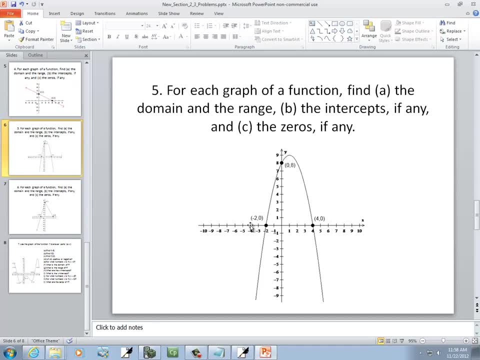 Domain is your x-values, where your graph exists. Well, if I come out here- I know this is kind of small- If I come out here to negative four, if I go down, I don't see my graph right here, but this is going off, so the implication is it keeps going forever. 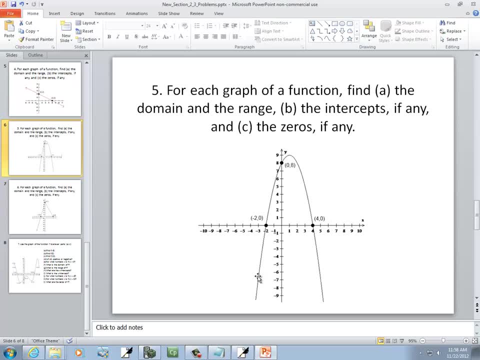 So, as it keeps going forever, see how it's slowly going to the left, Which means it'll keep slowly going to the left until So it goes to negative infinity. This, as it's going down, is slowly going to the right. 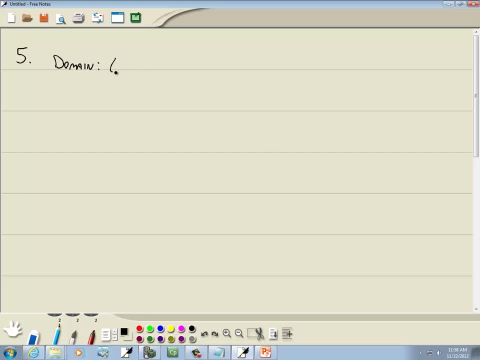 So it'll go to positive infinity. So our domain is negative infinity to positive infinity. Now our range is our y-values, where our graph exists. Well, it's going down forever, so it's obviously going to negative infinity. This is the high point of my graph. 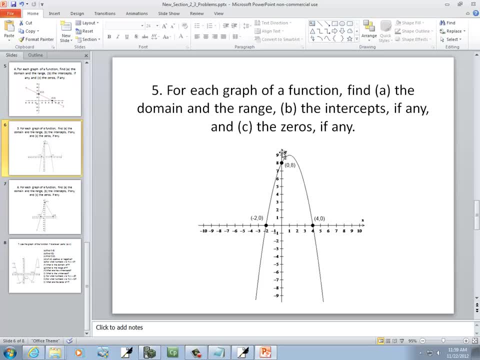 So that's the highest part of my graph. So if I go over that's at, y is equal to nine, So it goes up to nine and then stops And bracket on the nine. The intercepts: The x-intercept is where it touches or crosses the x-axis, which is negative, two zero. 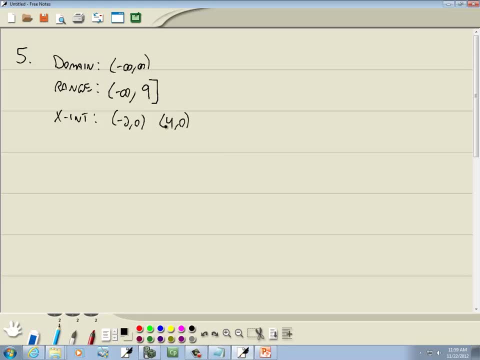 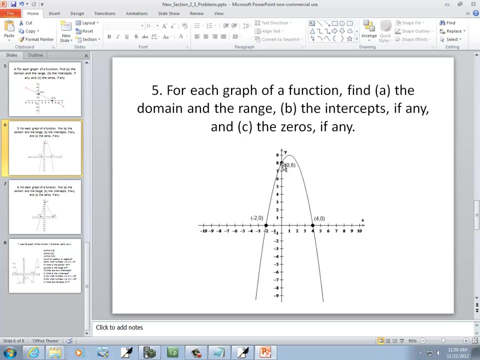 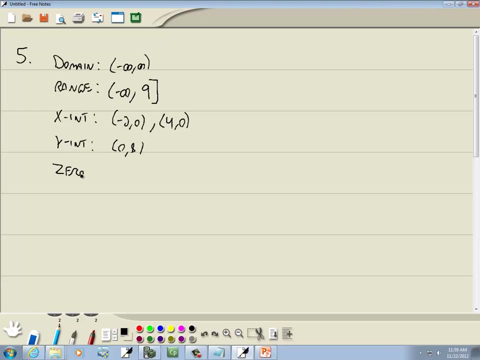 And four, zero. Now, our y-intercept is where it touches or crosses the y-axis which is up here, which is zero. eight, And our zeros is where it touches or crosses the x-axis, which is negative. two and four: 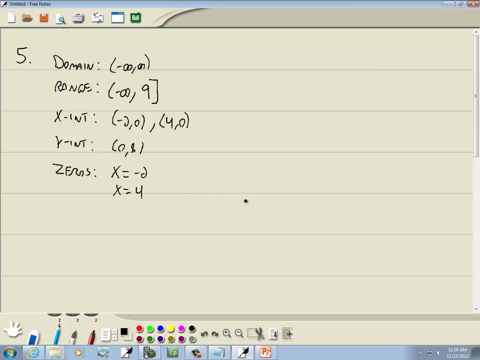 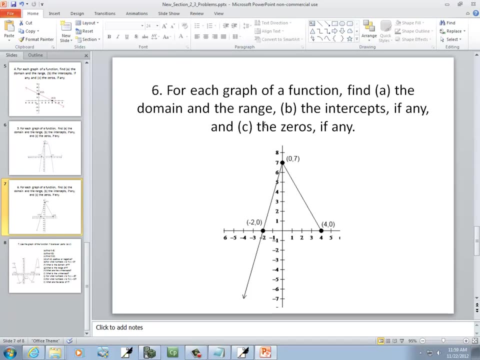 So we'll have: x equals negative two and x is equal to four. Let's look at number six. Same instructions, It says for each graph: find the domain and the range. Domain is your x-values- where your graph exists. Well, this is as it's going down. it's slowly going to the left. 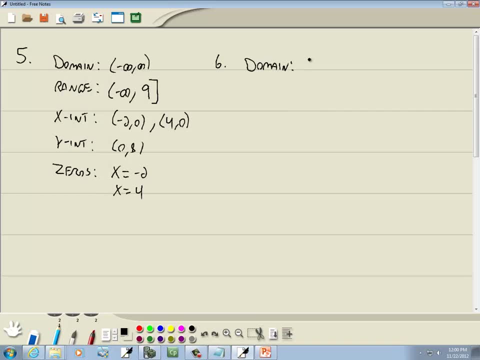 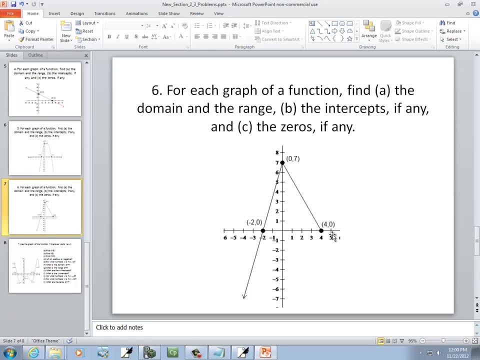 So it's eventually going to keep going to the left, which means this goes to negative infinity. Now this dot right here means our graph ends there. So if I come to, x equals five. if I go up or down, I don't find my graph anywhere. 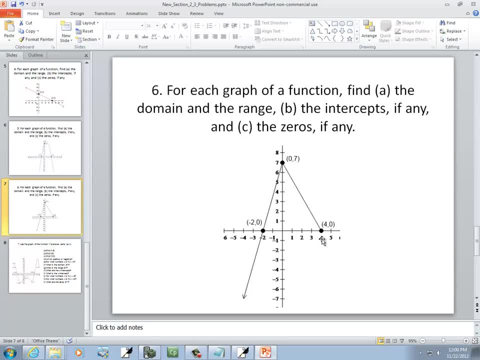 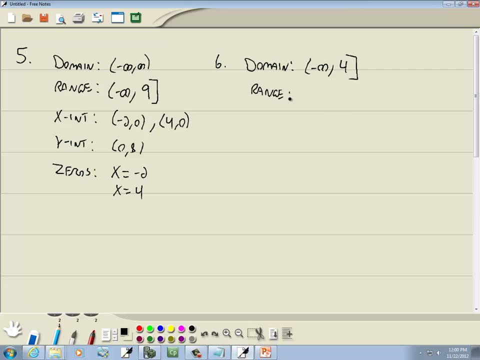 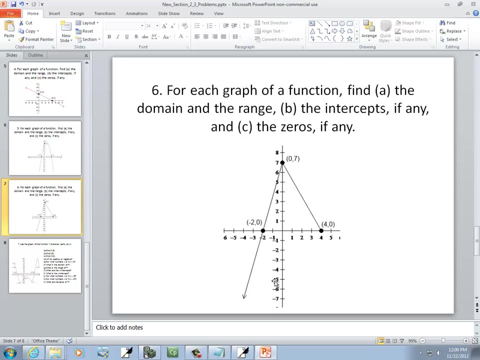 Actually the rightmost x-value where my graph exists is four, So that goes to four and then stops. Now our range is our y-value, So it goes down forever, which means it encompasses all the y-values going down. 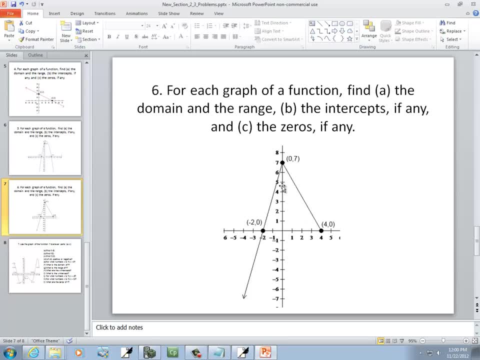 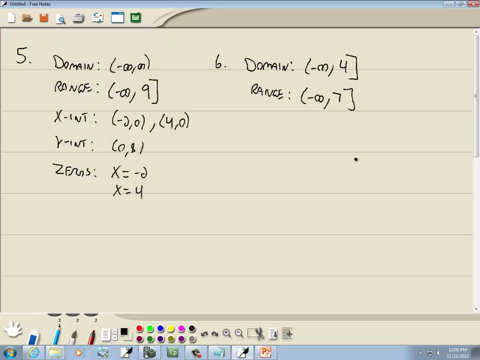 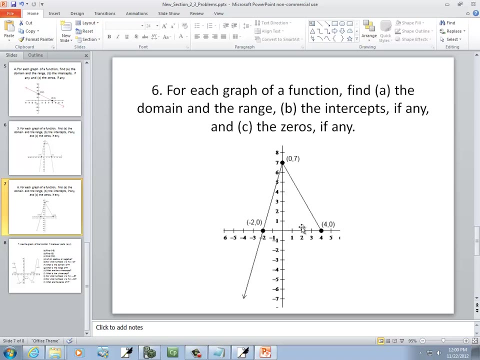 which means negative infinity. Now, our highest point where the graph exists is right here, And y-value-wise that's seven. So it goes from negative infinity to seven x intercepts where it touches or crosses the x-axis, Which is negative, two-zero and four-zero. 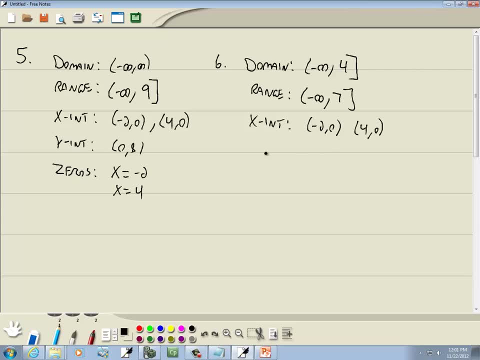 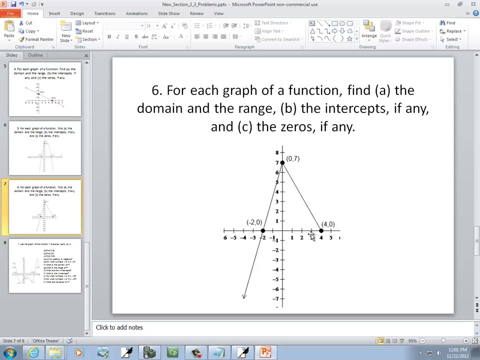 So negative two-zero and four-zero. Our y-intercept is where it touches or crosses the y-axis, which is zero-seven. Our zeros is where it touches or crosses the x-axis, which is negative two-four. And again, we write this as: 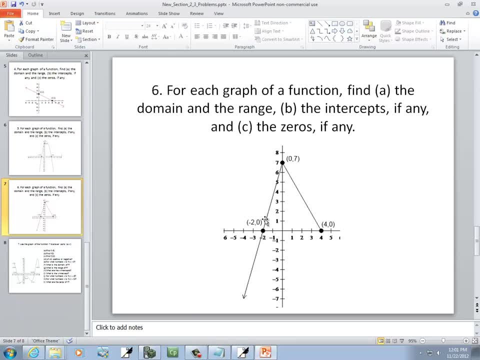 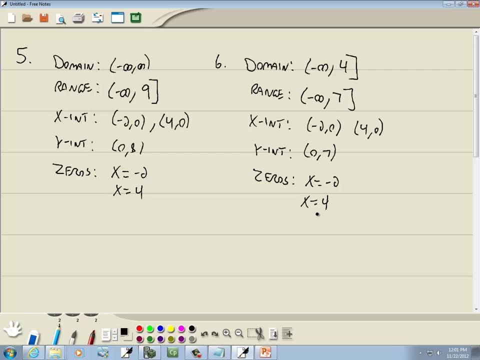 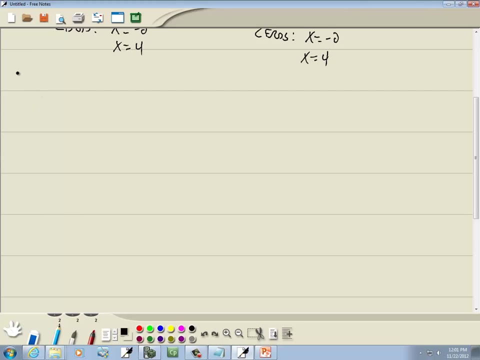 That's weird. Is that the same as the last problem? Negative two-zero, Sure enough, I'm not very imaginative. there am I. It should be those. It's not always negative. two and four, if you're wondering. Now, number seven introduces a new idea. 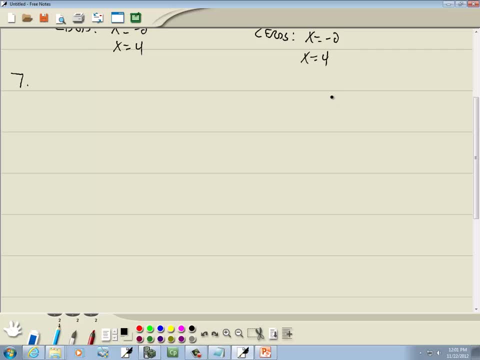 So let's talk about it. If you got f of some kind of number Equal some other number, Like that Number inside the parentheses, This is going to be your x And the number on the other side will be your y. 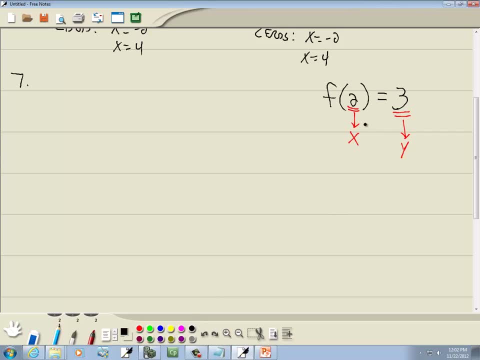 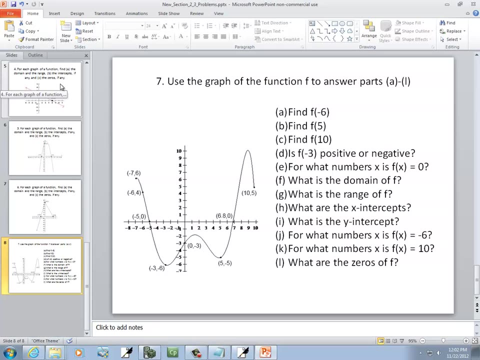 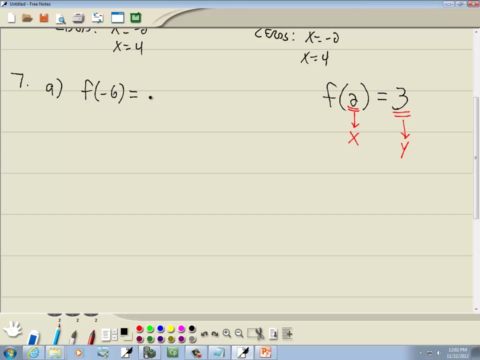 That's what a lot of these problems revolve around. is this idea right here? So again, whatever's inside your parentheses is your x, And whatever's on the other side is your y. Now a here says we want to find f of negative six. 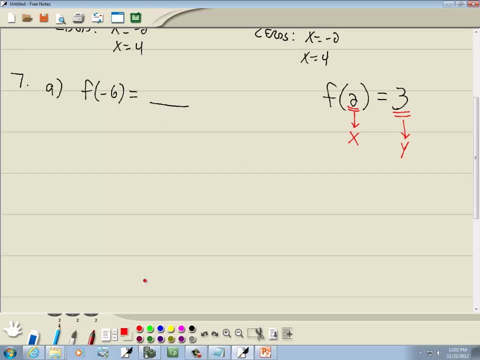 Given the graph. Remember what I said: Whatever number's inside your parentheses is your x. Basically, we're saying x is equal negative six And this is your y. So we're wondering what y is. So we're going to go to the point on our graph. 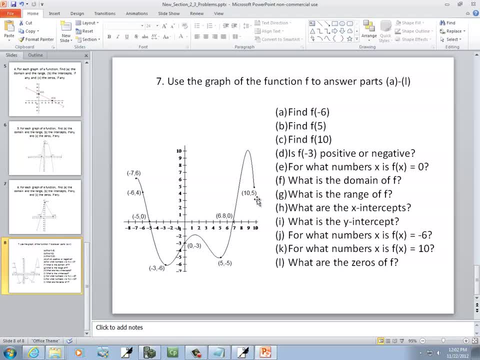 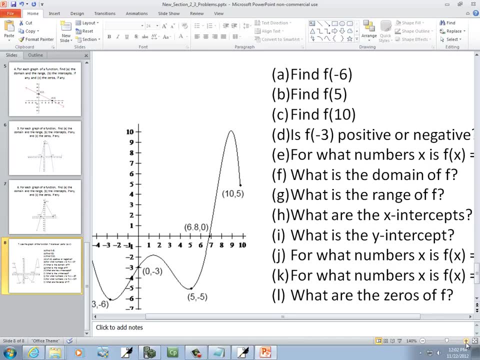 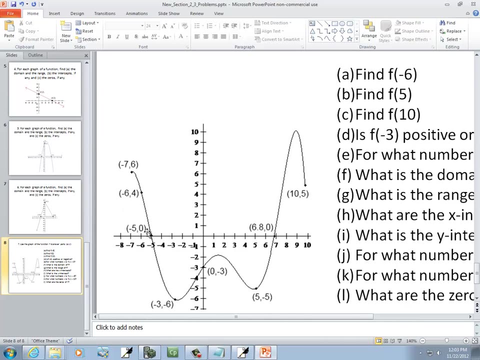 where we got x equals negative six. Well, Let me make this a little bit bigger So you can see it. Well, here's negative six On my x axis. If I go up, then this is the point where my graph is equal to negative six on my x values. 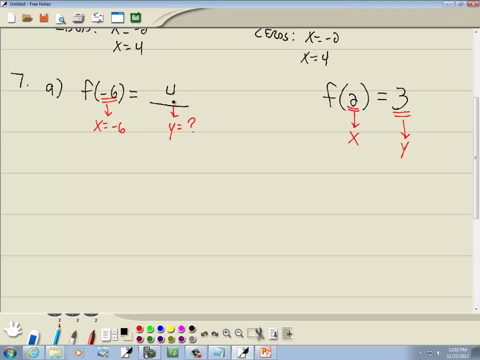 Well, if I look at my y value, it says four, So our answer is four. So basically we're just looking for the point on our graph where x is equal negative six and then writing down our y part. Now b says: find f of five. 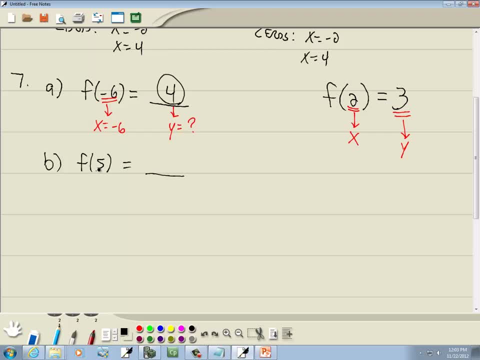 Again, what's inside the parentheses is your x. So they're telling us x is five And they're wondering what y is equal to. So we're looking for a point on our graph where the x part is equal to five. Now here's: x equals five. 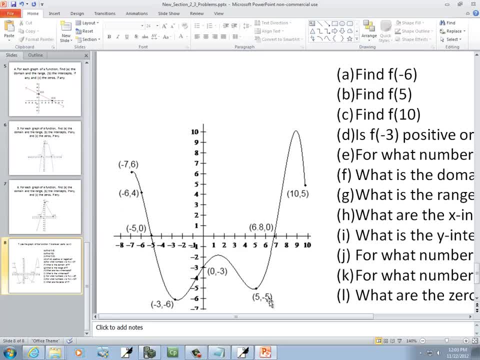 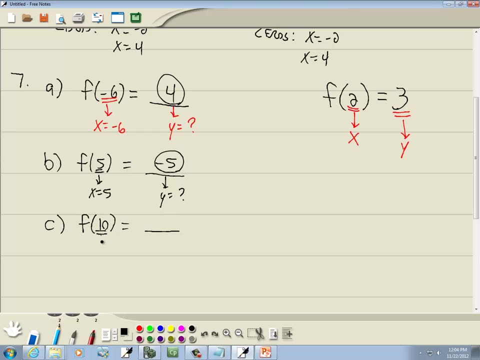 If I come down to here, here's my point. This is five negative five. So our y part is negative. five C says find f of five. C says find f of ten. Again, this is going to be our x part. 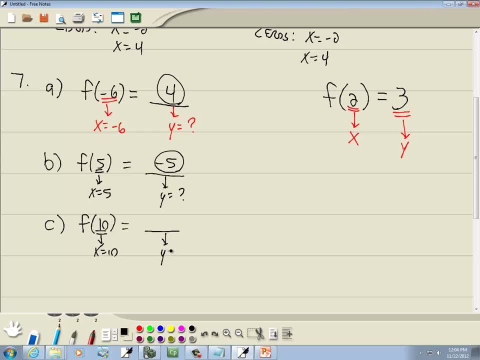 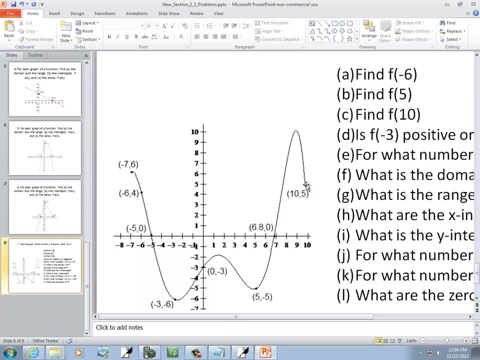 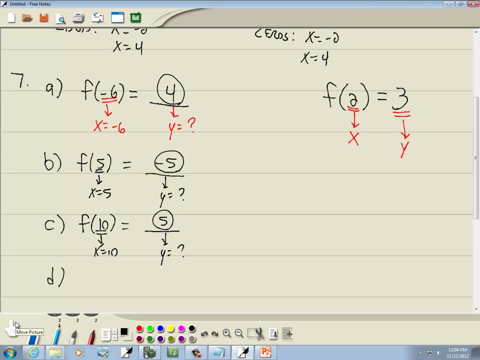 So we've got: x is equal to ten And we're wondering what y is equal to. Now, if I come over here to x equals ten, if I come up to here. here's our point. Our y part is five. I'll grab a drink here. 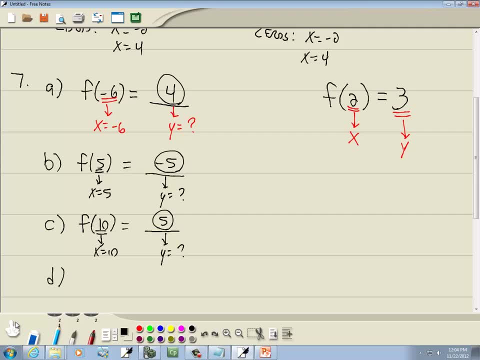 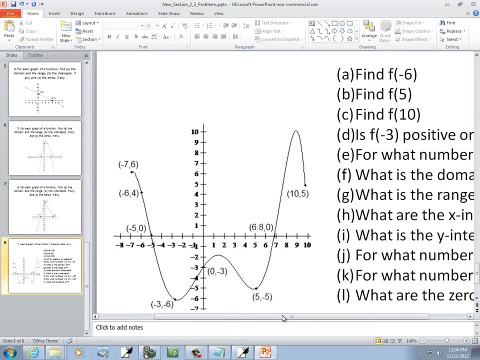 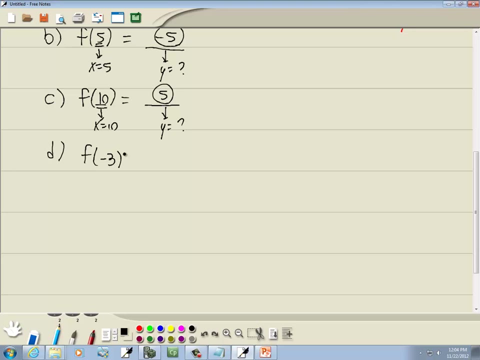 Okay, D says: is f of negative three positive or negative? Well, let's just find out what f of negative three is, And then we can go from there Again. what's inside the parentheses is our x. So they're telling us x is negative three. 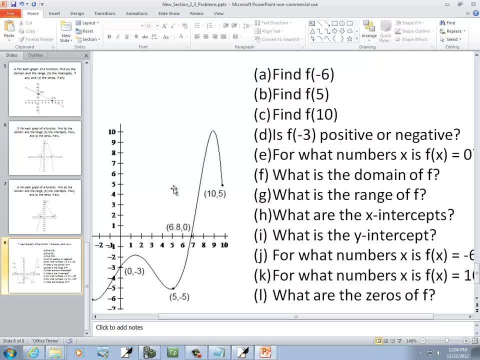 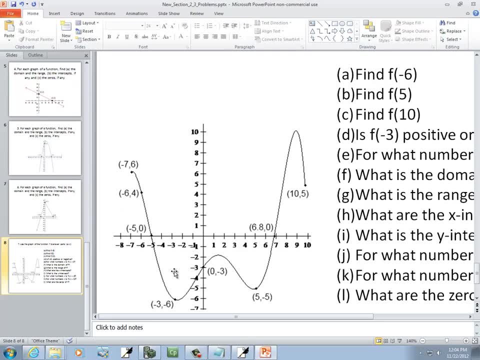 And we're wondering what y is. So let's go back and look at our graph. where x is equal to five, Well, negative three. Well, here's negative three. If I go down, here's where my point is. My y part is negative six. 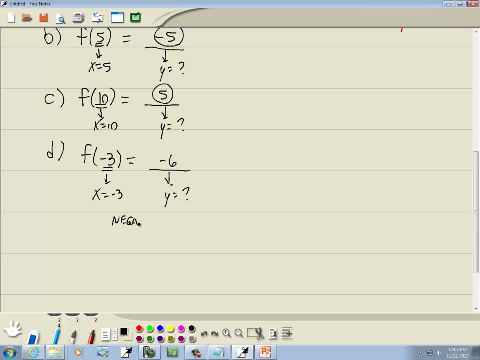 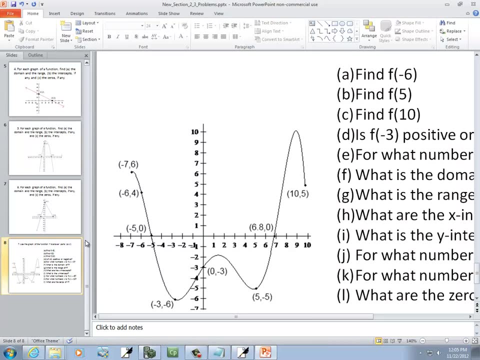 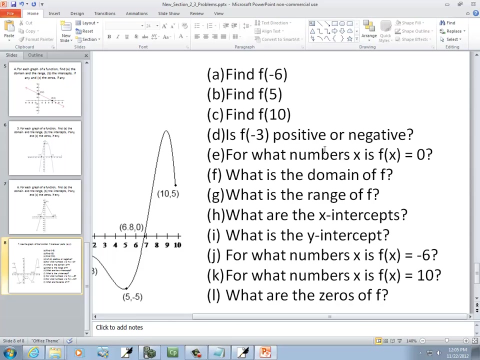 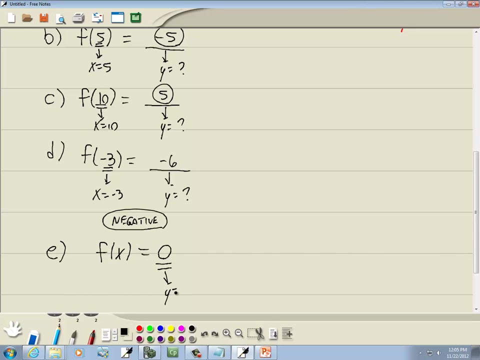 Well, negative six is obviously negative E. It says for what numbers x is f of x equal to zero. E, E, E, E, E, E E. What they're telling us here is they're telling us the y part. 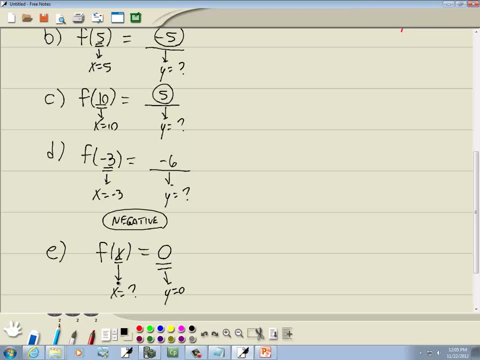 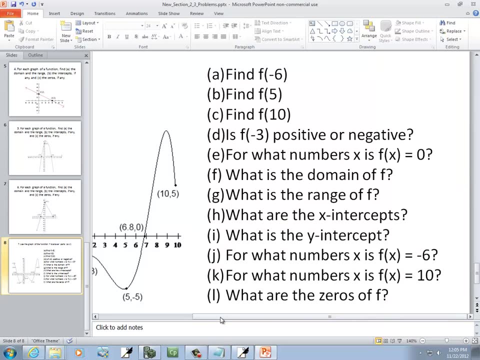 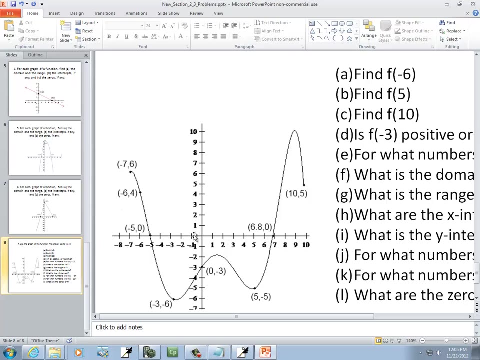 They're telling us y is zero And they're wondering what x is equal to. Now let's go to where y is equal to zero at. Here's y is equal to one. Here's y is equal to negative one y is equal to zero is right here, which is actually the x-axis. 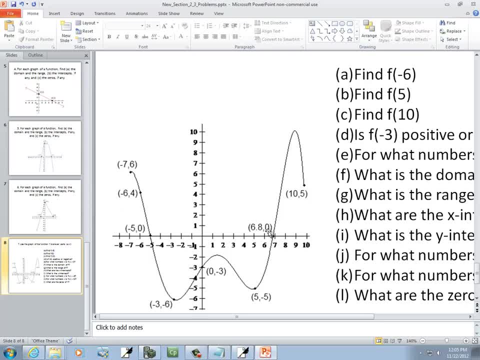 If I come over to here, this point right here has y is equal to zero And the x part is 6.8.. part is 6.8.. But if I come over to here, this part also has y is equal to 0 and the x part. 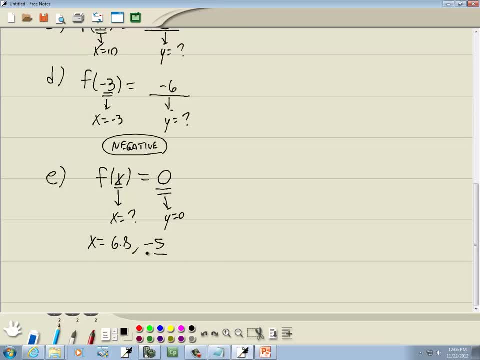 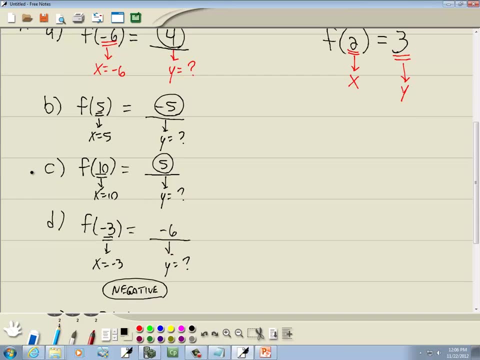 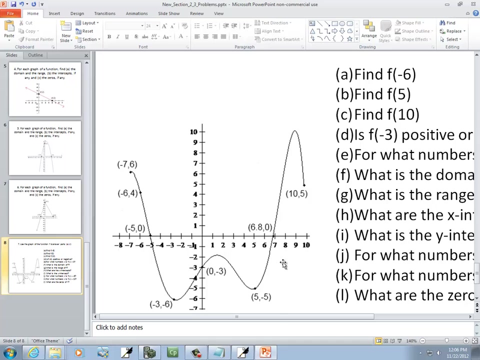 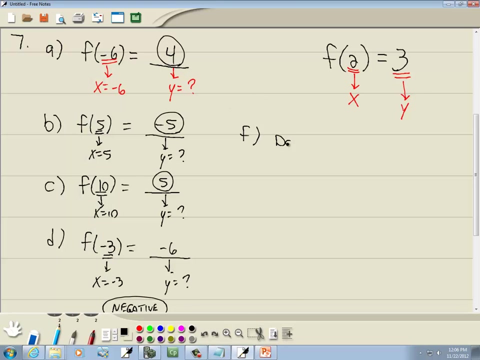 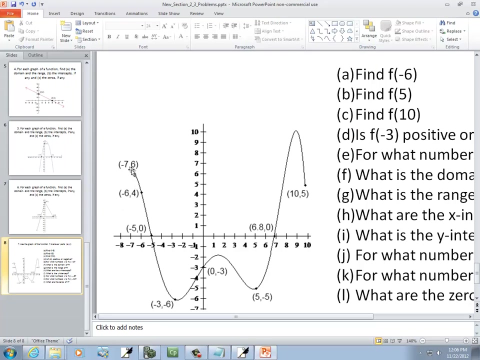 is negative 5.. So those would be our two answers for that part. So let's look at f. F is what is the domain? Yeah, So the domain, Remember. domain is your x values, where your graph exists. Well, this right here is our leftmost point. If I come straight down, then our x value is negative. 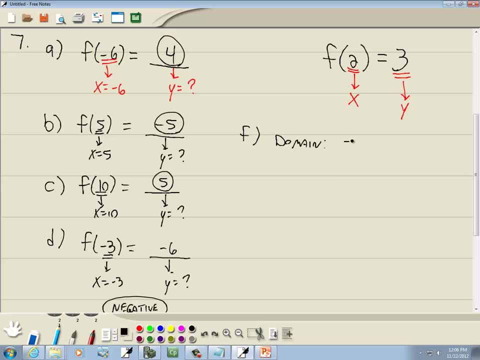 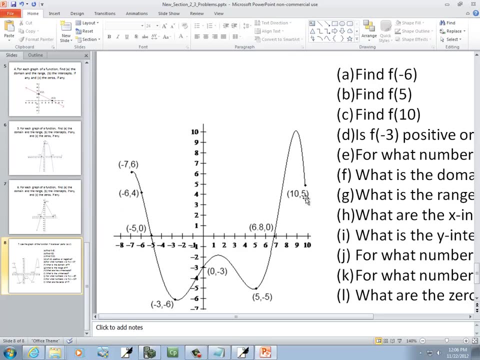 7. You can also get it off the point. So the negative 7 is the leftmost where it exists. Now here's the rightmost part of our graph where it exists. If I come down, it's 10, or I could get. 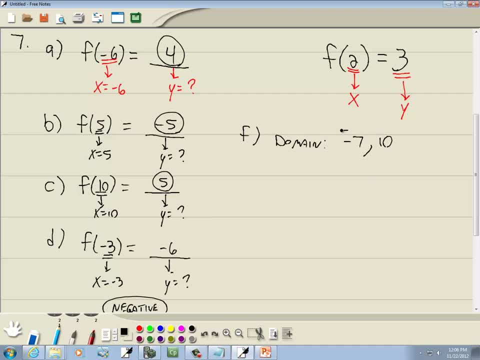 it off the point there. So it would be negative 7.. Negative 7 to 10 is our domain And we put brackets on those. Now our range is our y values, where our graph exists. Well, this right here is our lowest part of our graph. So if I come over, 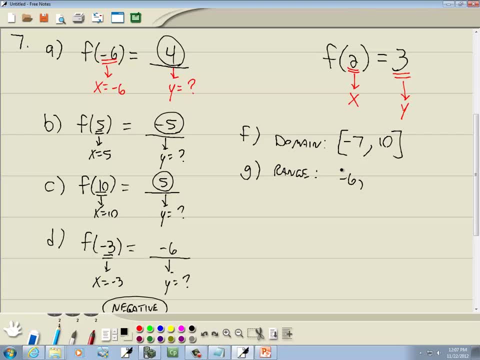 here it's negative 6. Because again, you're looking where your graph exists. Now this is the highest part of our graph And if I come over here it looks like it's 10.. So our range is negative 6 to 10.. 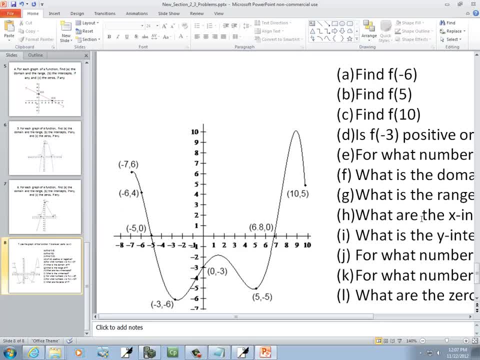 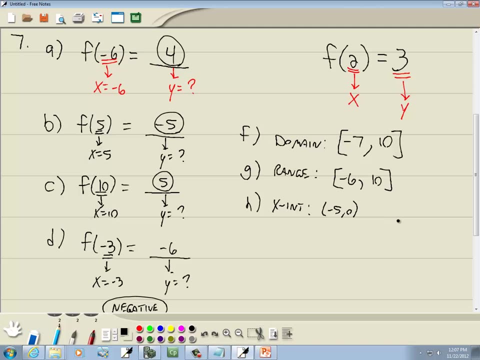 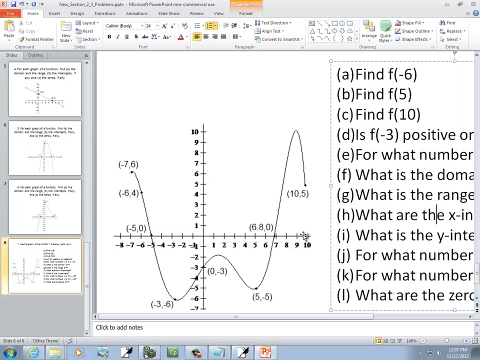 H looks like. what are the x-intercepts? X-intercepts is where it touches or crosses the x-axis, which is negative: 5,, 0. And 6.80.. And y was our y-intercepts And that's where it touches or crosses the y-axis, which is right here. 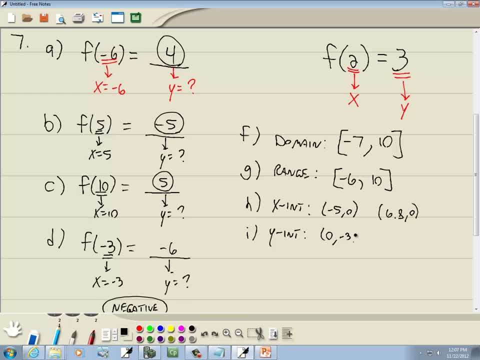 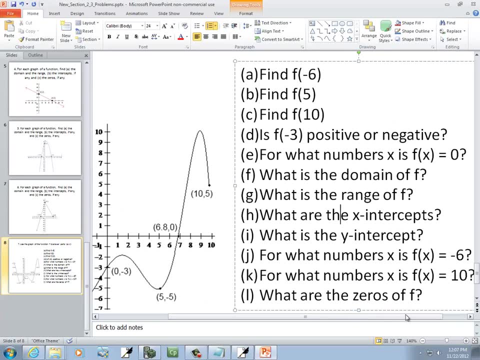 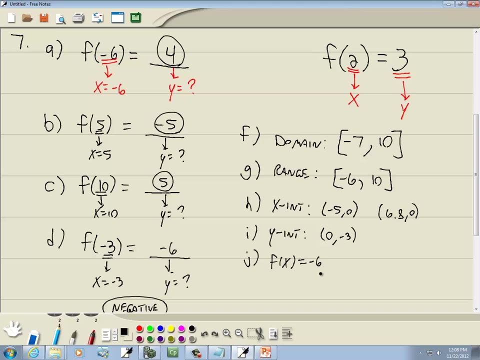 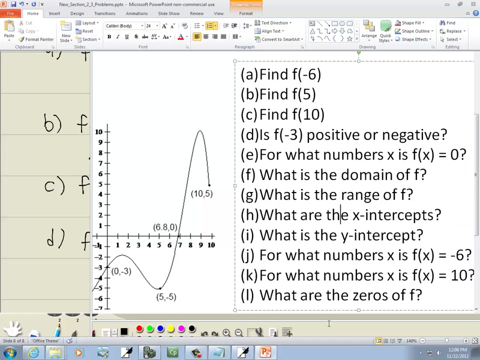 which is 0, negative 3.. J is what numbers? f of x is equal to negative 6?. Okay, so they're telling us here that y is equal to negative 6.. And they're wondering what the x value is? Well, here's negative 6.. 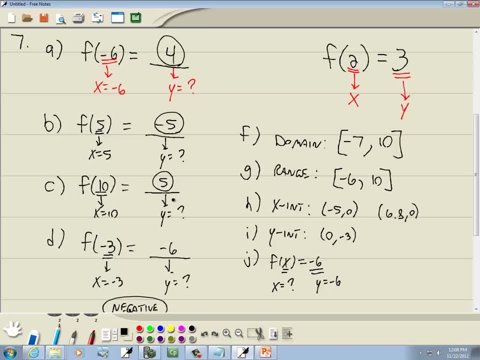 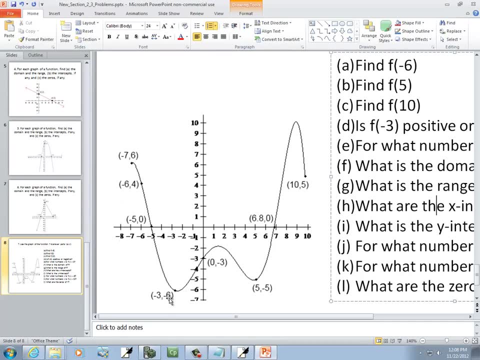 If I come up to here, here's my point. Wait a minute. y is equal to negative 6, sorry. So here's y is equal to negative 6.. So I come over here. this is where our y is negative 6, so our x-part is negative 3.. 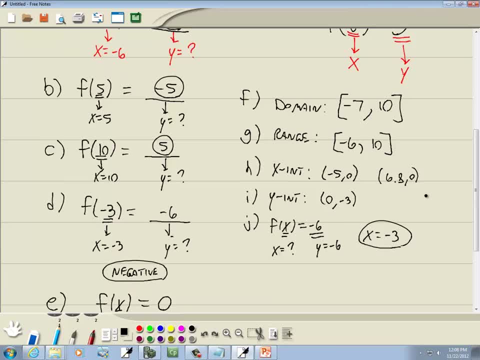 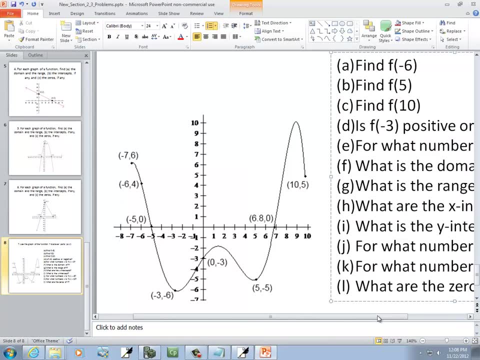 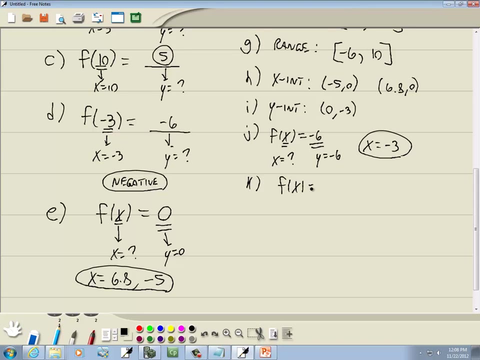 So x is negative 3.. Now k, I think, was f of 10. Or no, f of x is equal to 10.. So f of x is equal to 10, so here they're telling us the y-part, they're telling us y is 10, and they're wondering what x is.